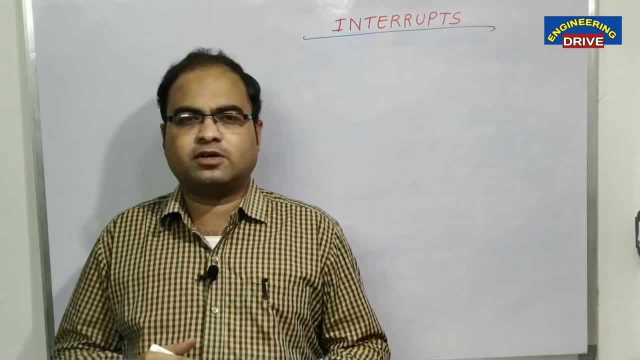 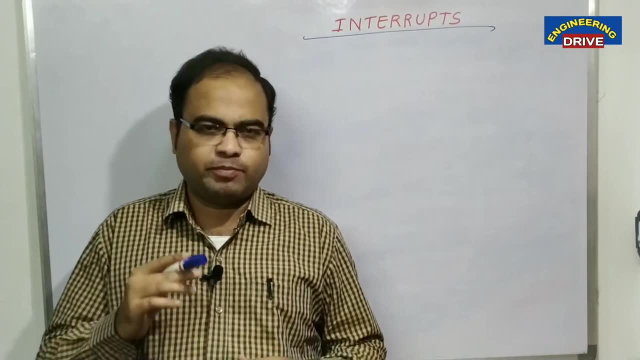 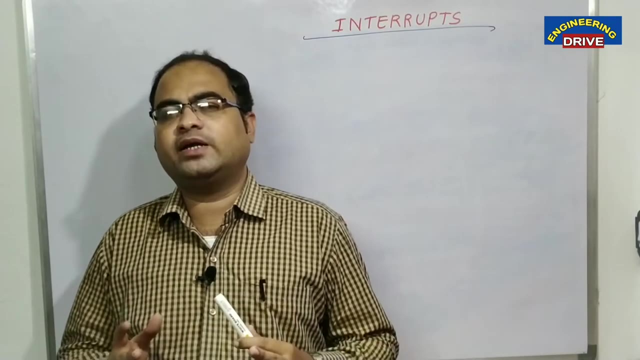 Sir, why there is a disturbance type of topic in CO subject, whether it is for the good sake of system. My dear students, whatever the topics we will discuss in computer organization, they are all part of only one requirement, That is, how we can able to develop computers with good performance. 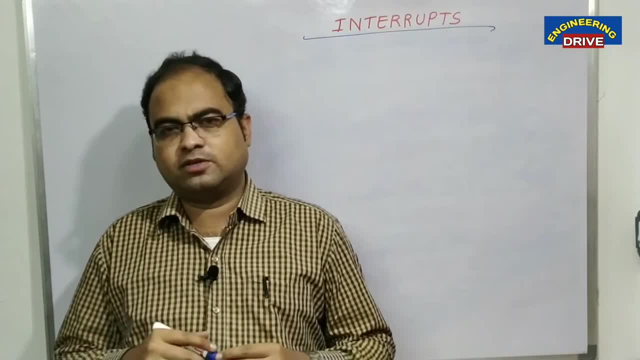 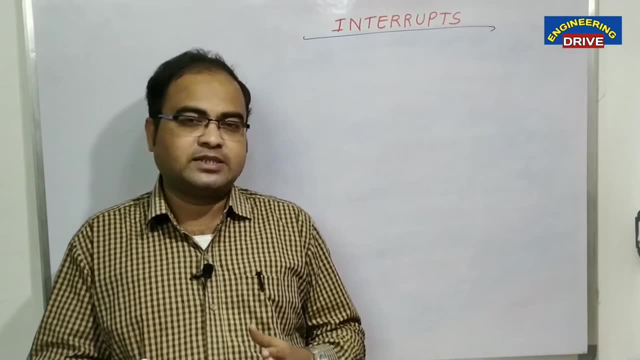 How we can improve the performance of computers, How we can remove the drawbacks of our system And at the same time how we can remove the drawbacks of our system. So with that sense we can able to guess that interrupt is also one of the added advantage of our systems. 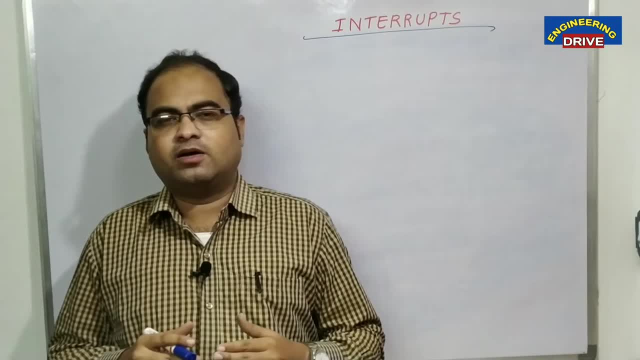 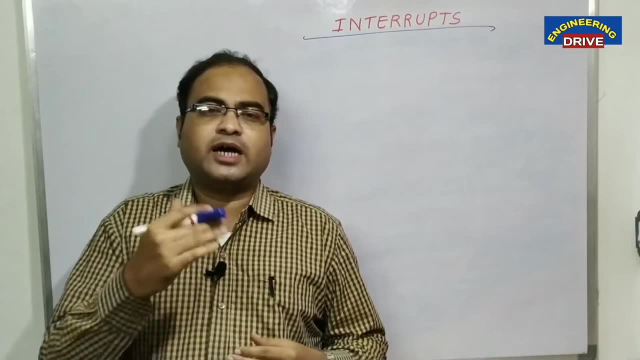 So what is an interrupt, Okay, why our computer will make use of this interrupt topic, and who will use this interrupt and what are the advantages, Each and everything I am going to clarify in my today's video. Okay, my dear students, 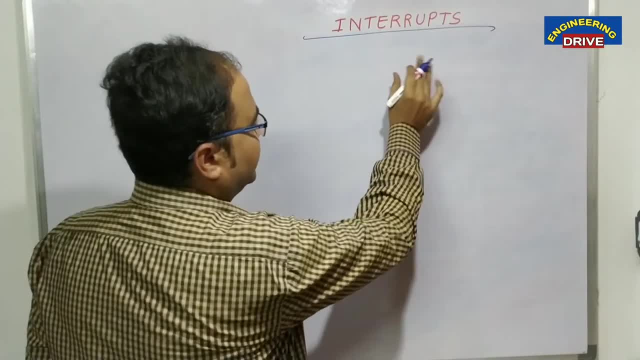 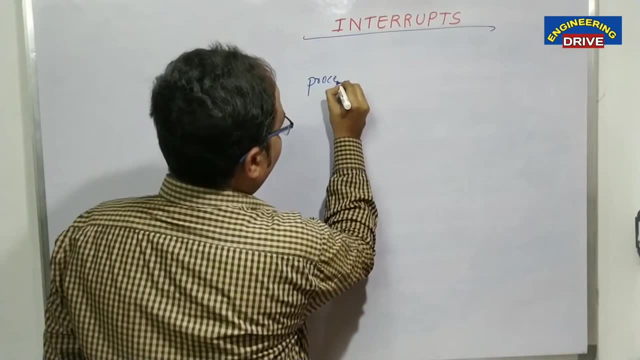 Let me tell you something. Let me tell you one scenario first, Then I can able to explain this interrupt with the help of one example, so that it will be clear to you. Let us say: this is our processor and here there is one output device, that is a printer. 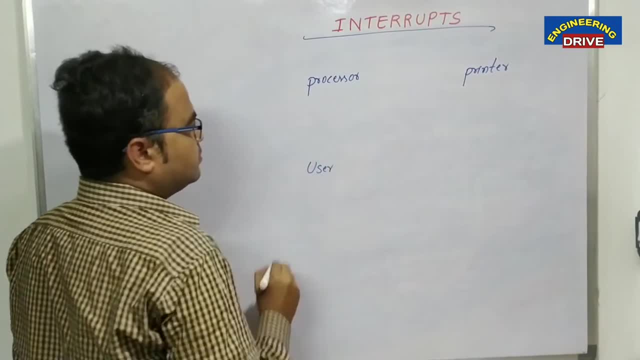 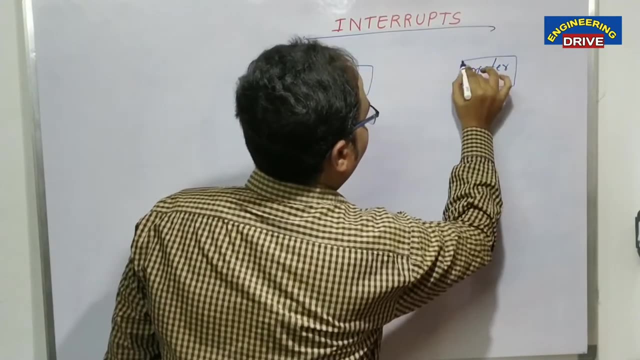 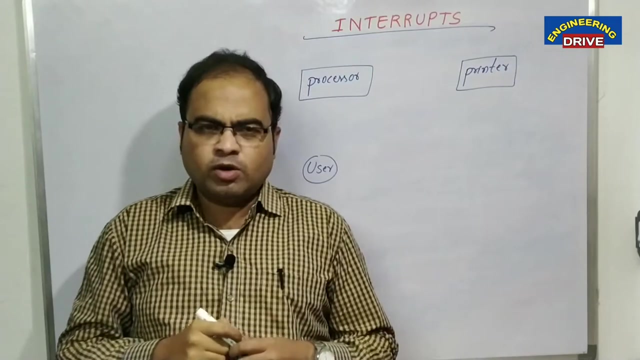 Okay, and this is a user. Okay, this is a user. this is our processor and this is our printer: Output device, processor, user. So for our simplicity, I have taken only these three diagrams. Now let us say: user want to take out some prints of pages. 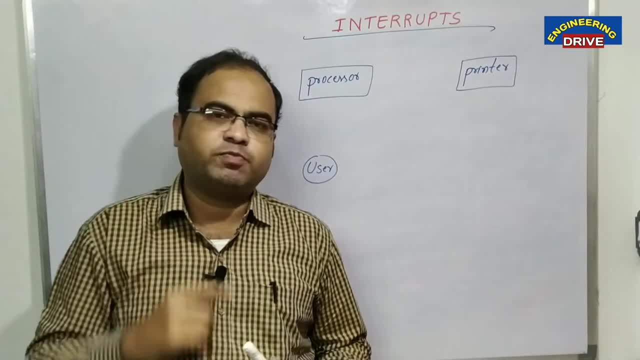 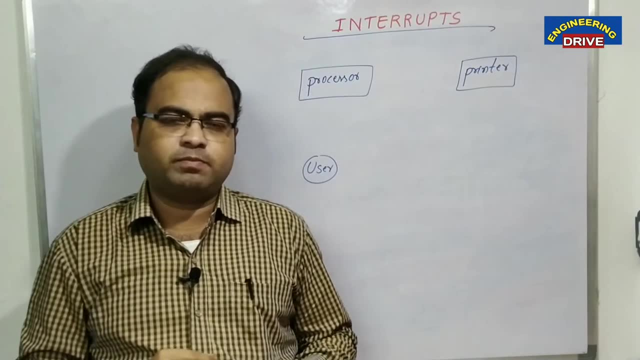 Let us say user want to take out 100 pages of print. How many 100 pages at a time? user has given the print command With the help of print command. user has given the prints Now. first, the request will go to the processor. 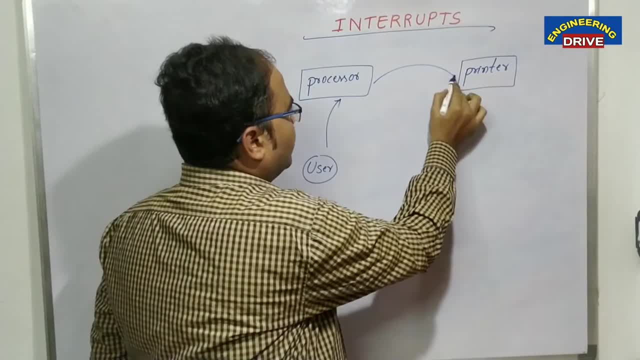 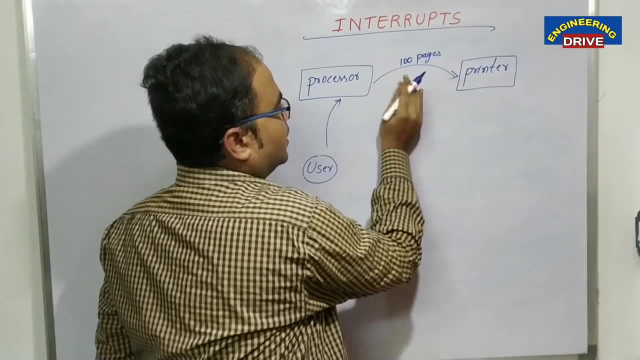 Okay now, with the help of processor permission, only the control will go to the printer output device. Okay now, with the help of processor permission, only the control will go to the printer output device. Okay now, this 100 pages command will go to the printer. and you know that printer cannot print those 100 pages within 30 seconds or 1 minute. 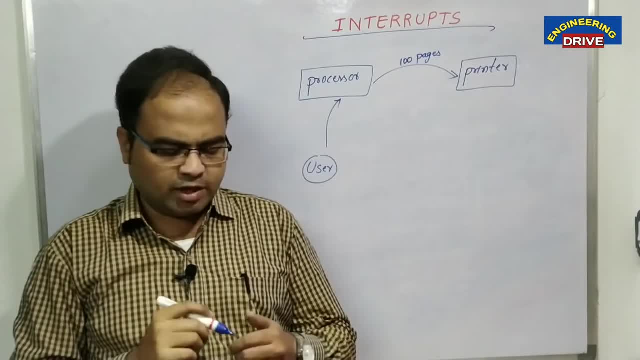 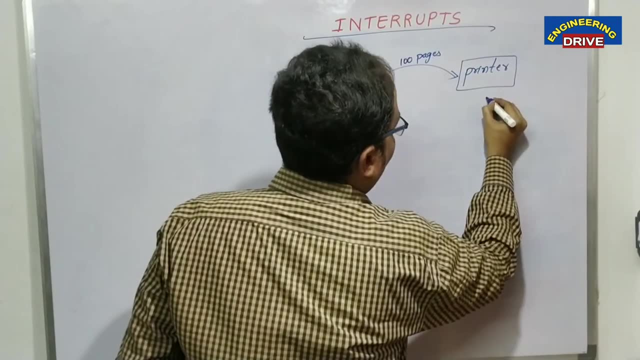 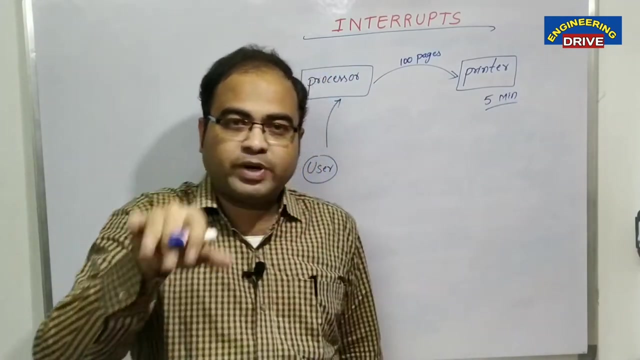 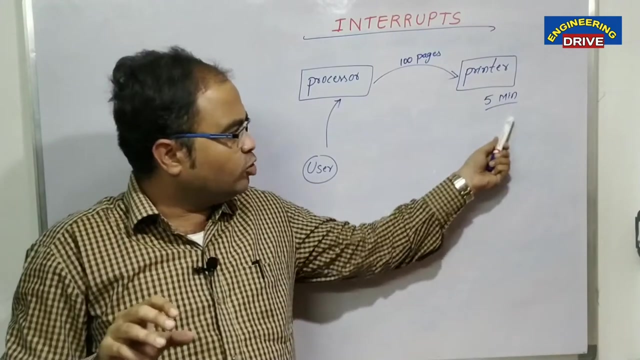 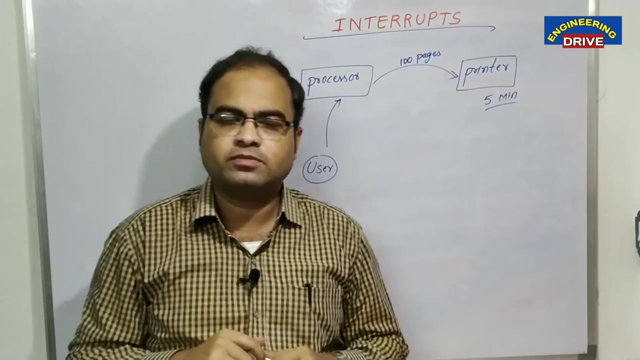 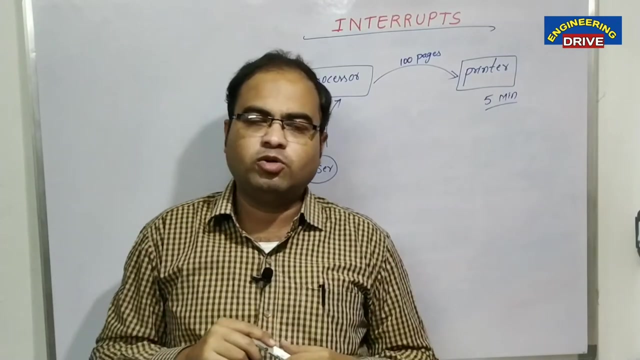 It is a matter of some duration, Yes or no, Depending on the printer speed. let us take this printer will take to print this hundred pages five minutes. How long it will take five minutes to print all those 100 pages. Okay, now what happened When the printer is printing those 100 pages in the duration of 5 minutes? during this 5 minutes time, our processor will be idle. It will be very free, which means it won't have any other work to do. Simply, it will be concentrating on when this 100 pages is going to finish out. 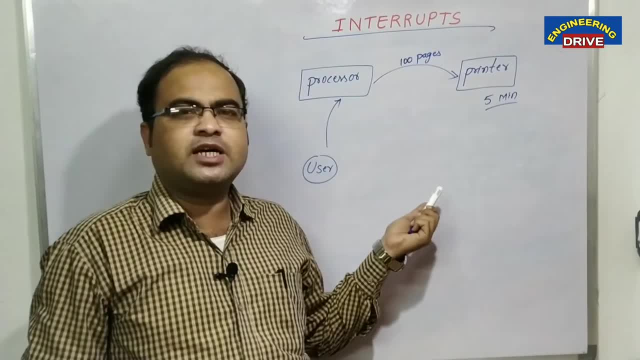 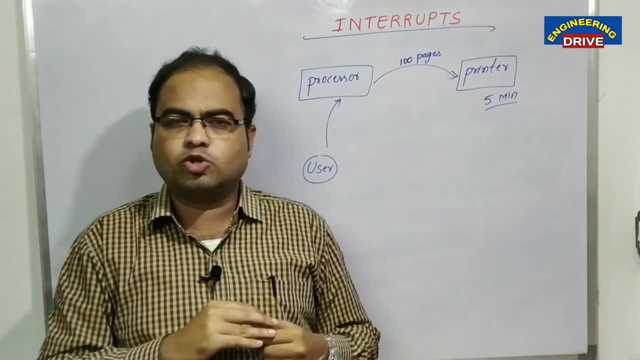 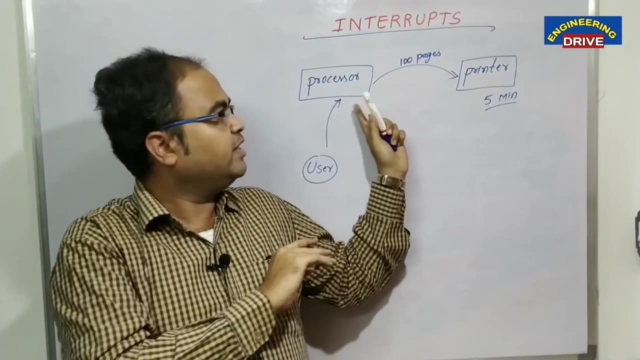 Okay, yes or no. Meanwhile, there will be some other device which wants the request of the processor, which wants the service to be fulfilled by the processor. So what we can do now, in this situation, We want to utilize our processor, but our processor is very idle. It is waiting for the 100 pages to get print Already. this work is going on. 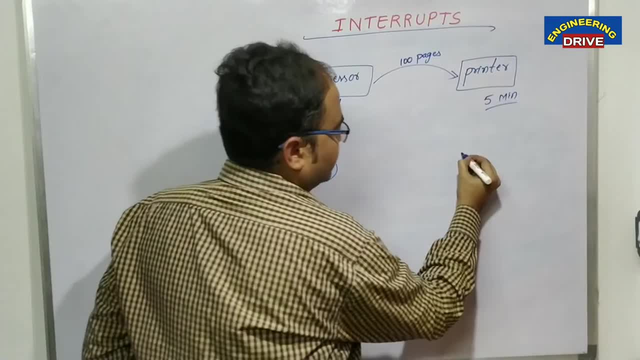 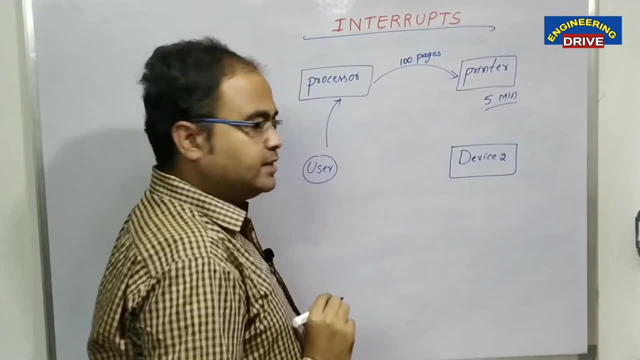 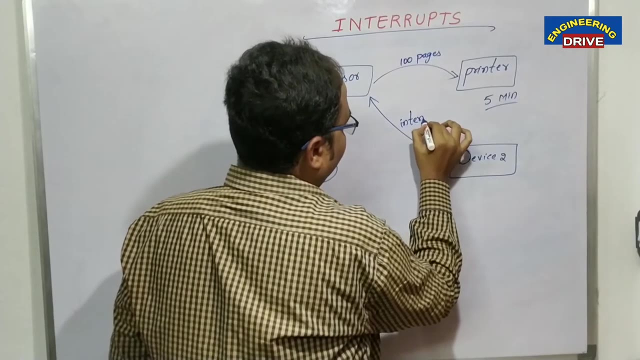 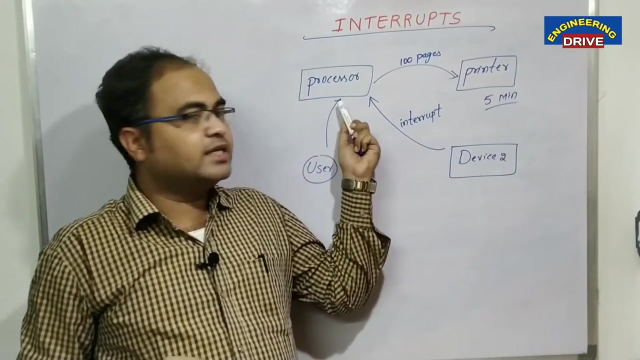 So what we can do, Let us say there is one more device, Device 2.. This device 2 also wants the request, Request of this processor At this time. what this device 2 can do means device 2 can send one signal, which is known as interrupt. It is a hardware generated signal. What signal it will send? Device 2 will send the signal directly to the processor. 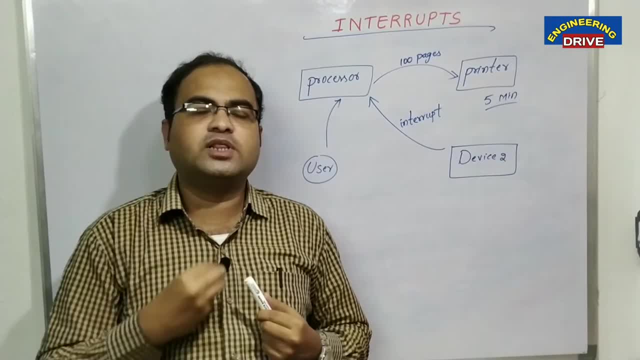 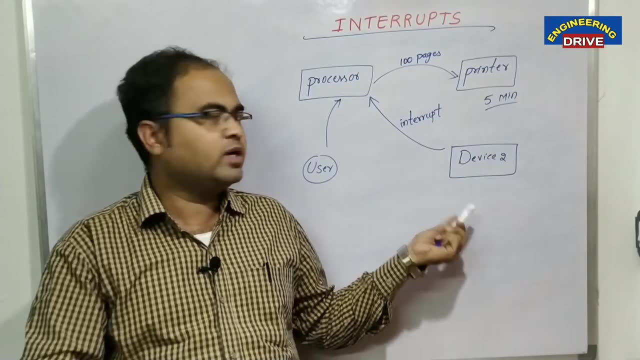 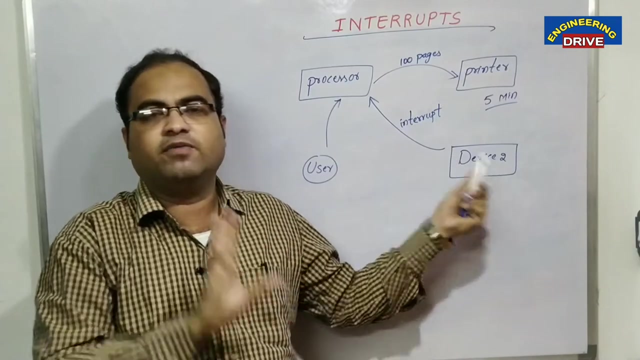 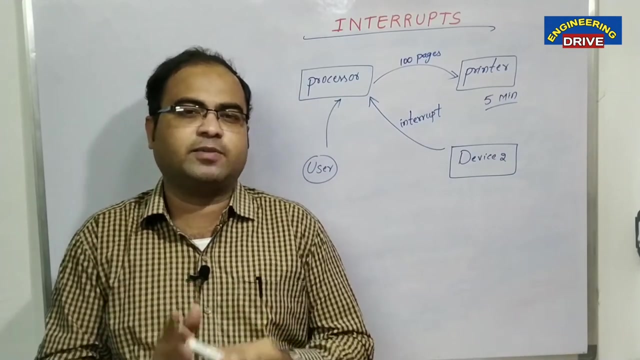 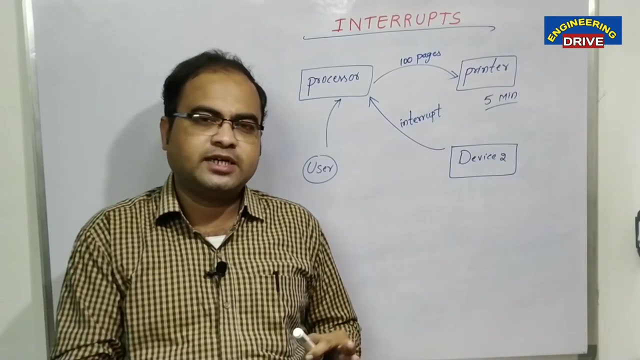 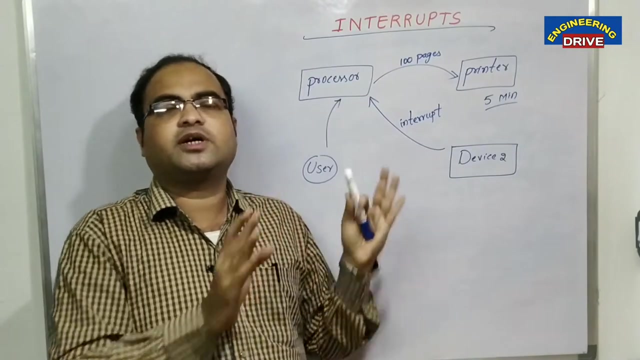 Yes, dear processor, I am ready to fulfill the request. Okay, my request is there. Please fulfill my request. I am ready to do this work. I am ready for this work. Please fulfill my request. Please give the permission. Then, once the processor will get this signal, processor can fulfill the device 2 request also. So hopefully the concept of interrupt has been cleared to you, Why this interrupt is used. Interrupt is a hardware signal which is generated by the devices. When they are going to generate this interrupt, whenever processor needs to fulfill the request, they will send this interrupt signal to the processor so that processor can fulfill their request. 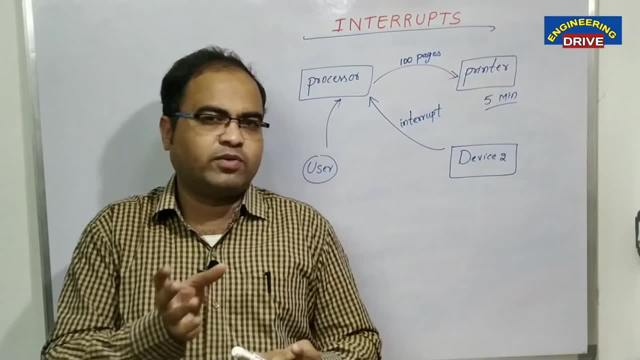 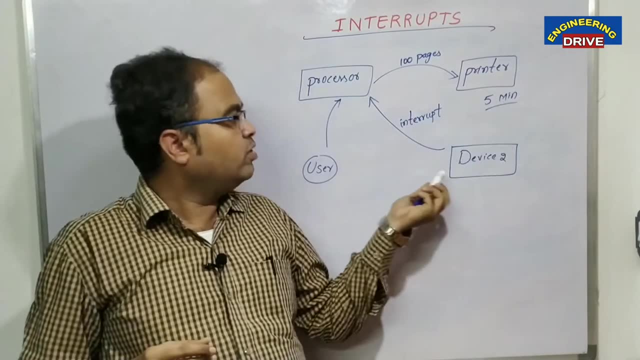 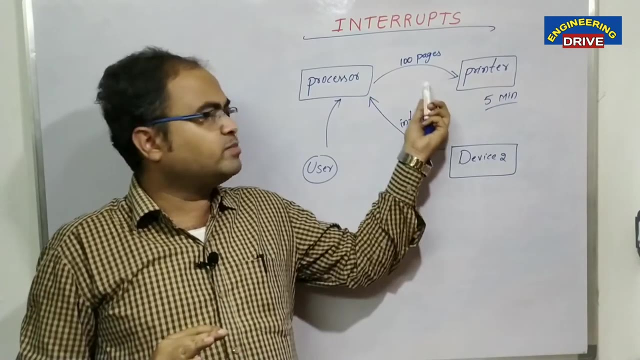 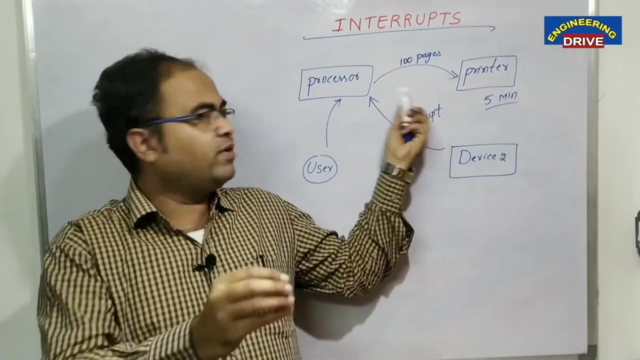 Okay, this is the purpose of interrupt. Why we are using the word interrupt. You know already processor is doing this work. What is that? 100 pages print, Even though device 2 has interrupted. Device 2 has interrupted the processor, for good sake only. Processor is idle, Only it is observing when this 100 page is going to print out, When these 100 pages are going to be printed. So meanwhile processor will fulfill the request of device 2.. Similarly it may happen for device 3, device 4 and so on. 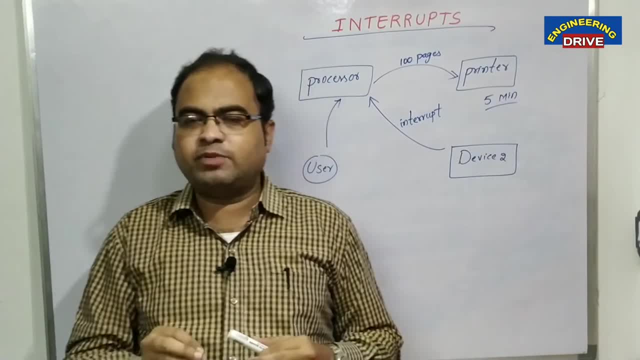 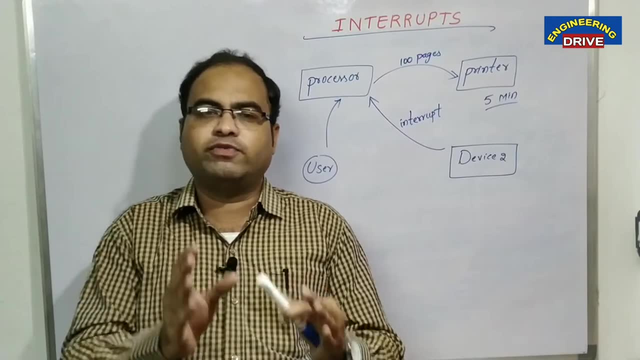 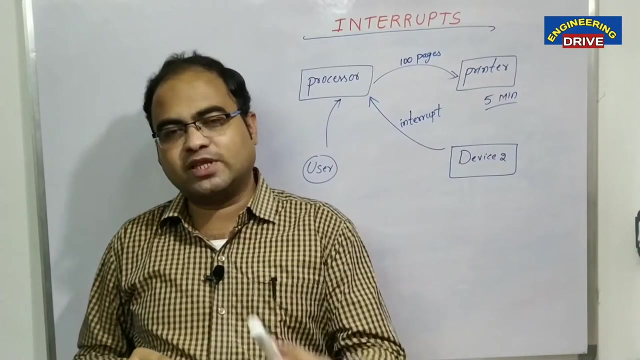 Okay, so what is a interrupt? An interrupt is a hardware signal. Who will generate this interrupt? Interrupts are generally generated by the devices Who want to fulfill the request And to whom the interrupts will be sent. Interrupts always will be sent to the processor so that processor can fulfill the request. 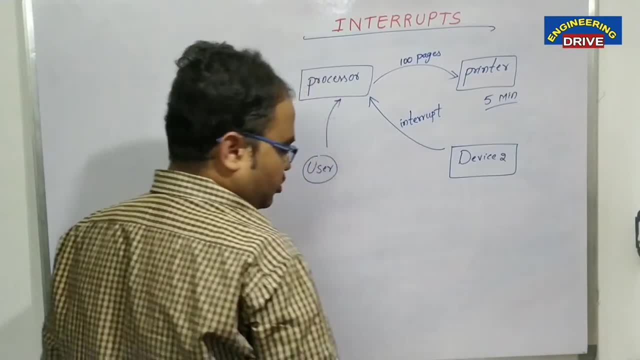 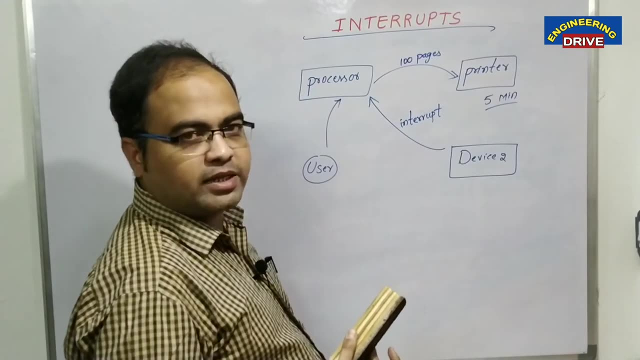 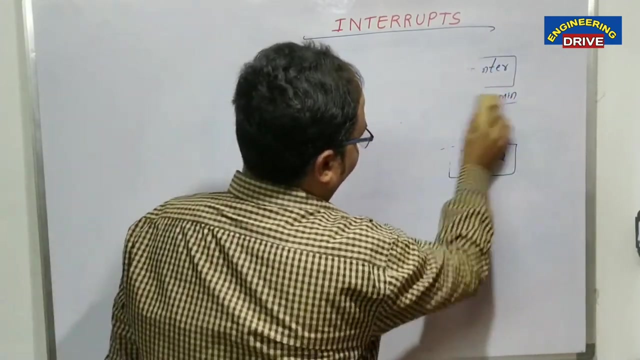 Okay, clear Now. let me take one more example to you to give the clear idea. So, if you want, you can take down this diagram See: simply pause the video and you can take the diagram. Okay, So online video lectures is: we will save lot of time. Okay, Students will save lot of time. A lecturer also will save lot of time, Yes or no? 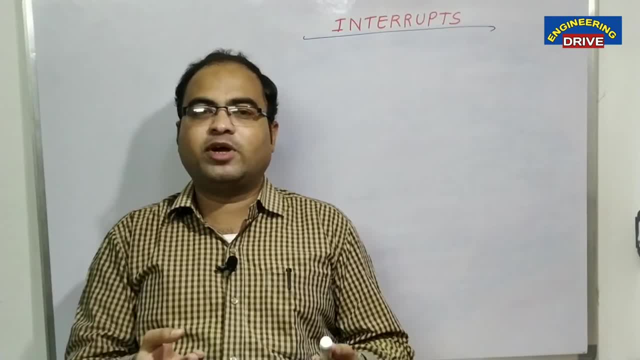 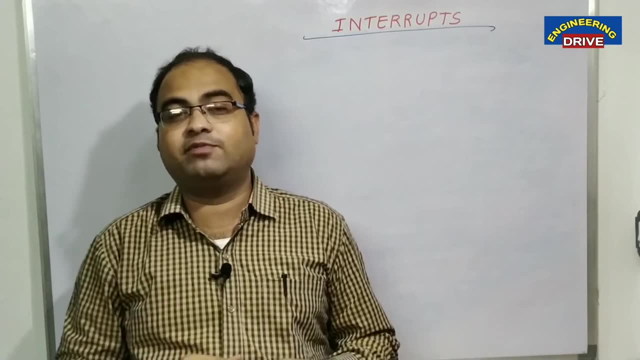 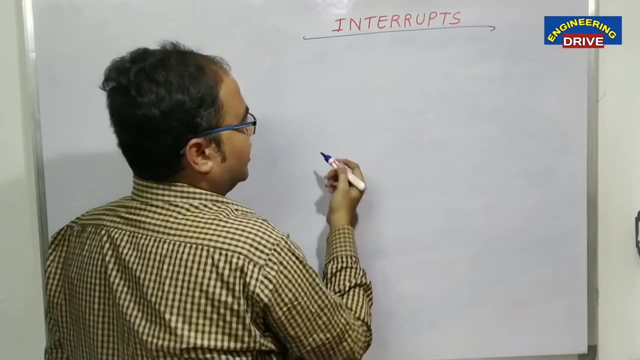 The reason behind this is because, simply, you can pause the video. There is no need for me to give separately, take 5 minutes and note down the or take the diagram, Yes or no. That is one of the big advantage of online lecture videos. Okay, Anyhow. so interrupts. Now let me take one more example. Let us consider there are two programs. 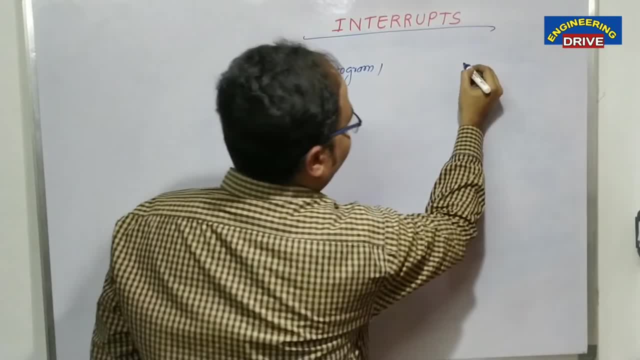 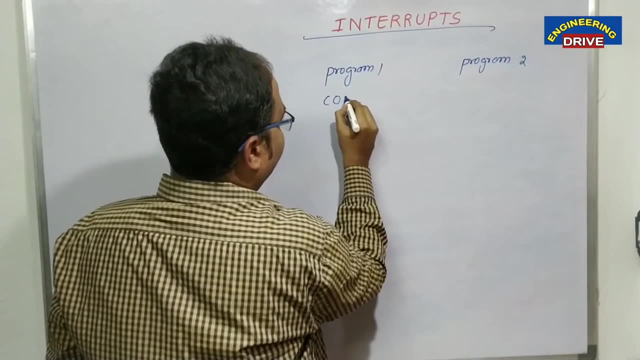 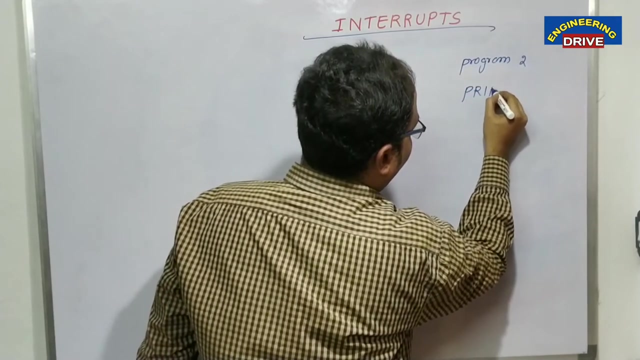 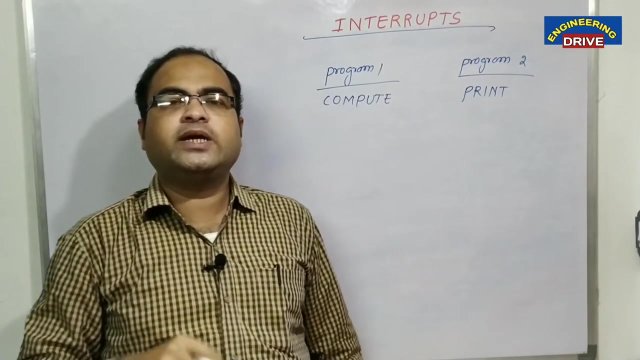 Program 1, and this is program number 2.. So this program 1 want to do this work Which work Compute work. Program 2 want to do this work: Print Compute program is responsible for producing lines of text. Some lines of text it will produce. 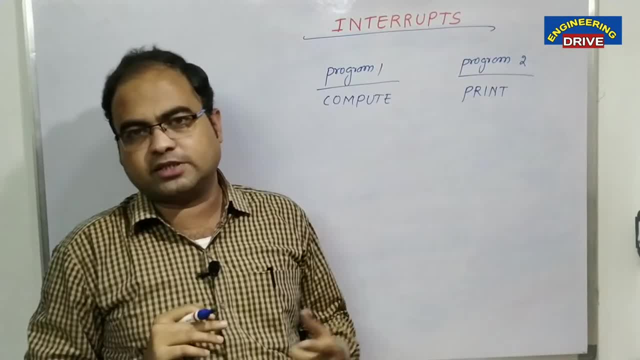 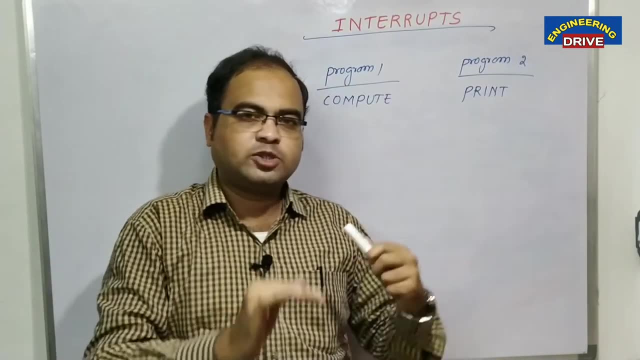 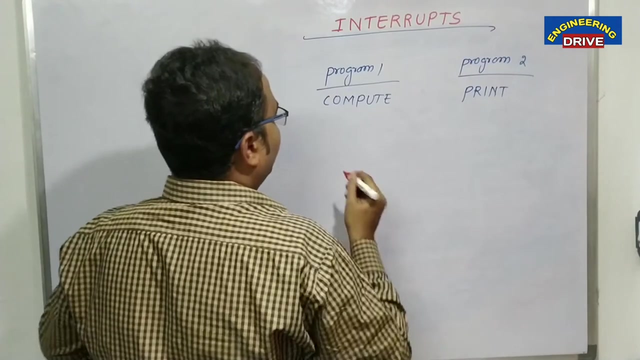 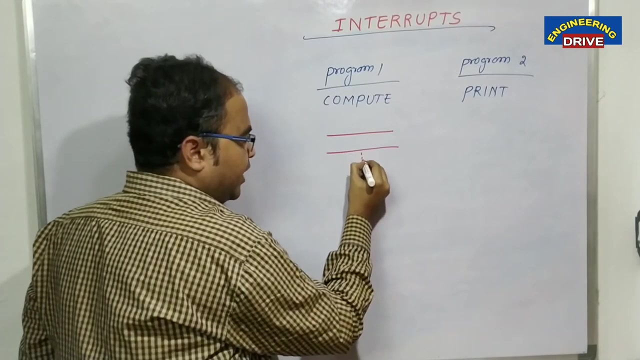 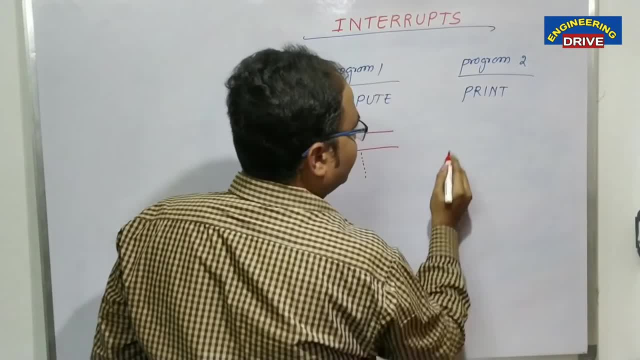 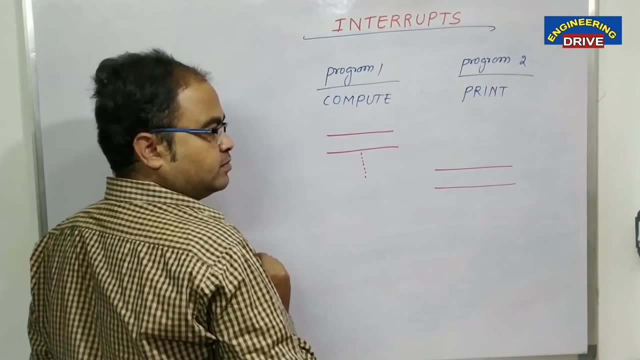 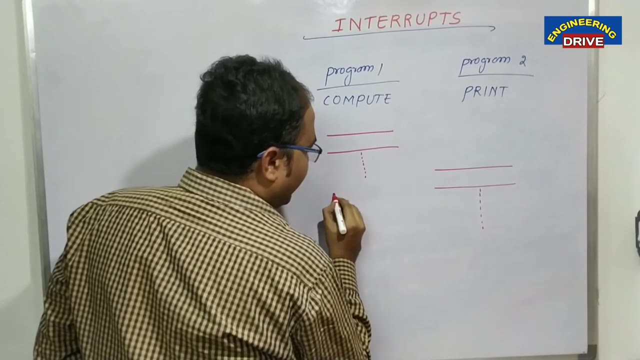 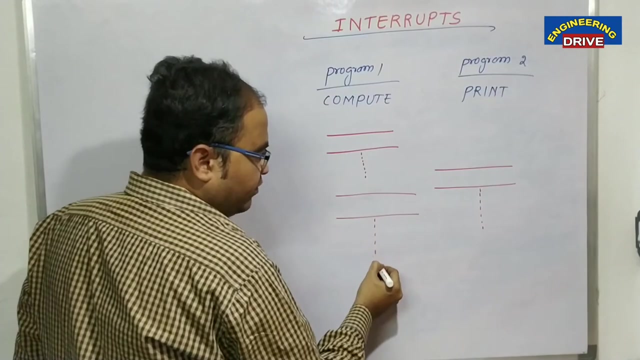 Print program is responsible to display this two lines attacking simultaneously. Okay Now, once it will display these two lines again, it will wait, Yes or no? During this waiting period, whatever compute program should do means it should generate these two lines of text. once it will generate this two lines of text again, it will go in waiting stage. 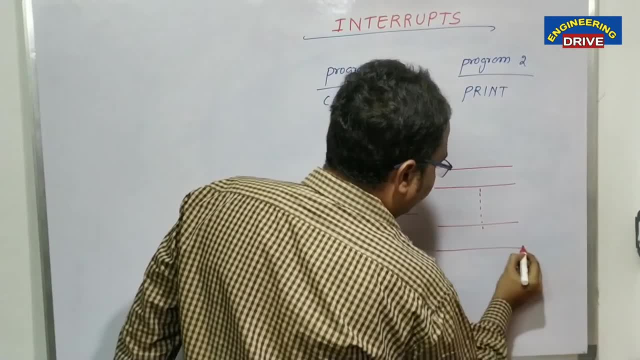 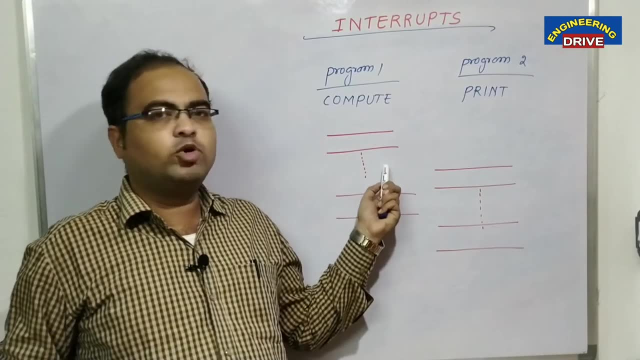 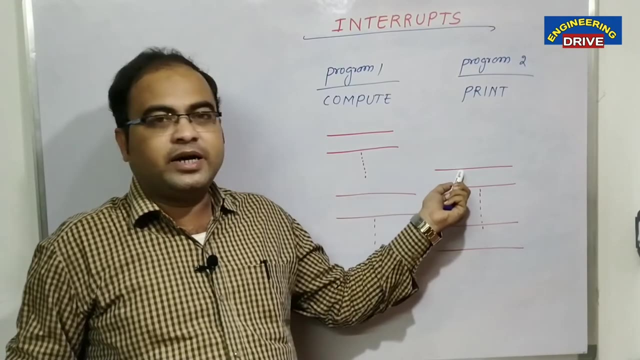 during this waiting stage. compute print program should print this lines of text, which means you got one clear picture here. when processor is busy in compute text, then what happened when the processor is waiting? it don't have any work during this time. the print program should utilize the. 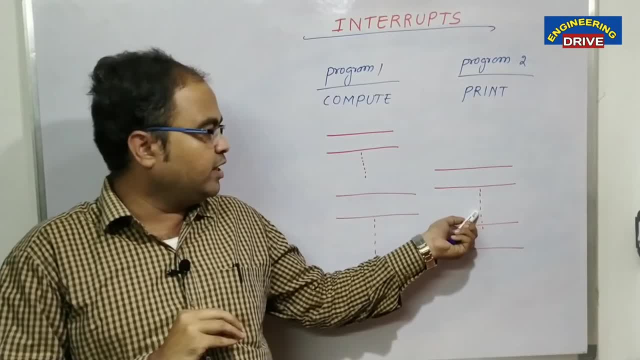 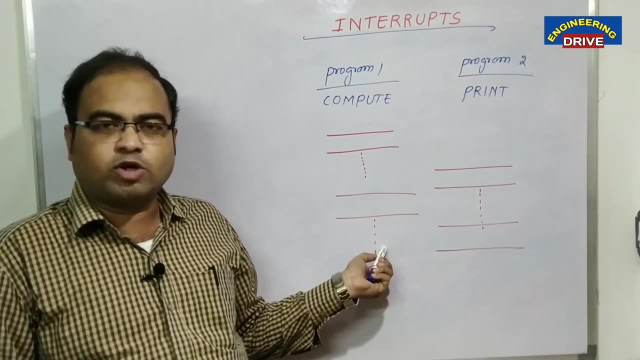 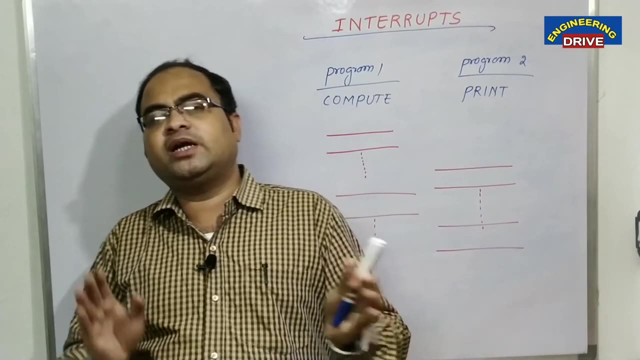 process. when the print program is idle, when it is not doing any work, the compute program should utilize the process. when compute program is free, when it is not utilizing the processor, then print program should utilize the processor. which means if one program is not utilizing the processor immediately, the other program should send the interrupt to the processor and it should take 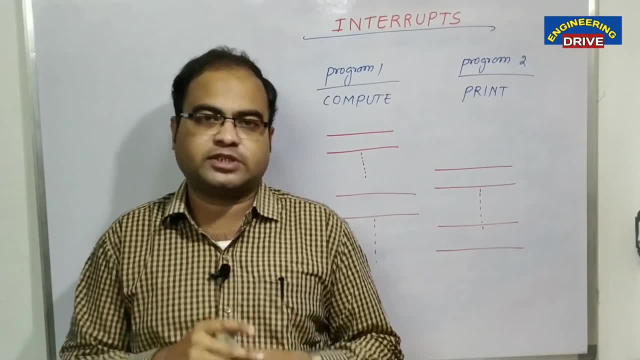 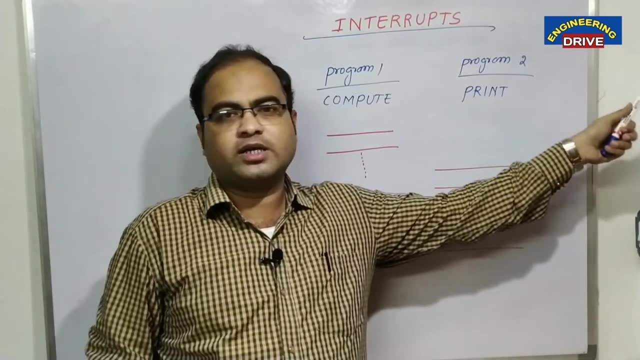 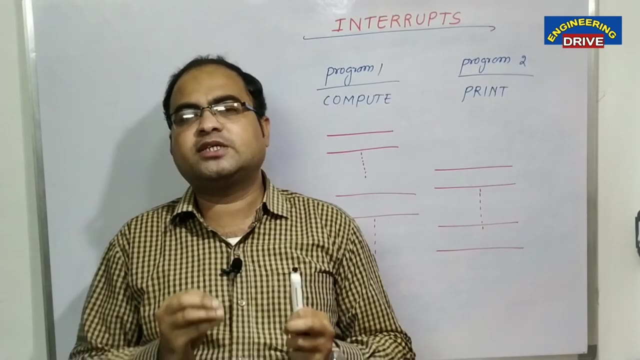 the permission from the processor and should fulfill their fulfill its request. that is the main purpose. that's why we have taken this example: compute and print. if you want, you can take one more program, program number three, which can do some other work. the main purpose of interrupts is the processors. idle time will be reduced with the help of interrupts. why? 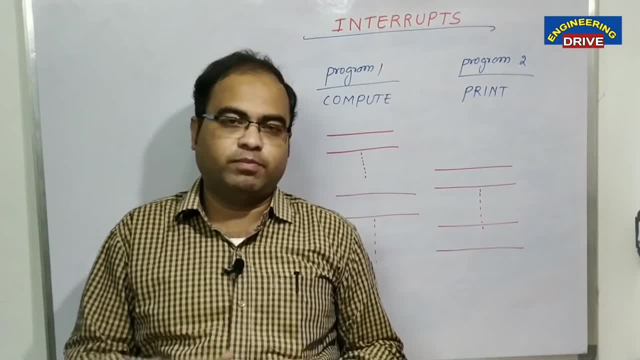 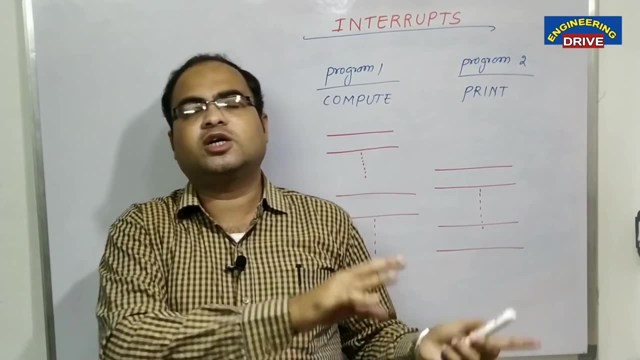 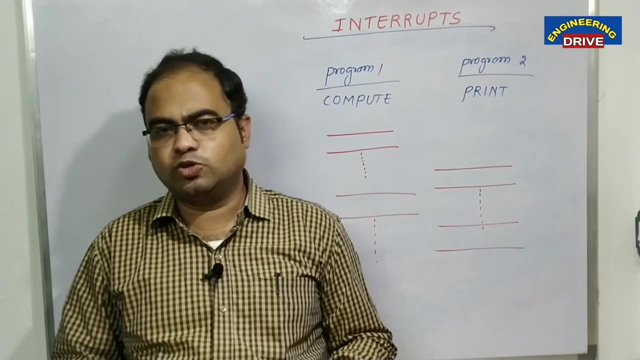 the processors. how the processors idle time will be reduced because of interrupts. if one device is ready to be get service immediately, it will send the interrupt to processor so that processor can fulfill the request of that device. okay, so hopefully the concept of interrupts has been clear to you.